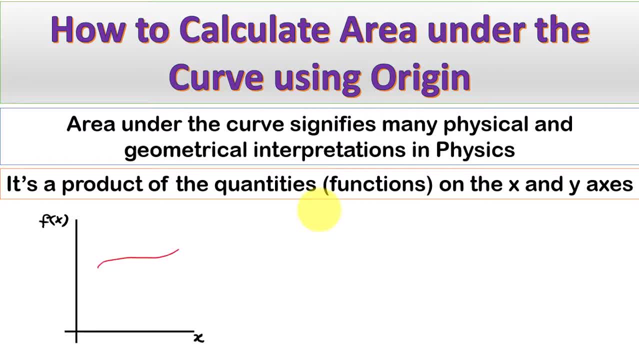 we consider a function f of x and the behavior is like this and we want to find out area under the curve of this function. Now, the desired area is this one and as we know that there is no fixed shape on which we can calculate this area, So the best approximation we will have to consider. 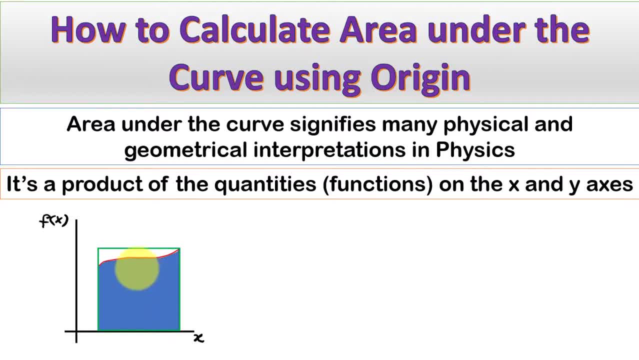 a rectangle on it and, as we know, that rectangle of side a and b is having the area a, b and in terms of f of x, i can write: the area is f of x multiplied by x. but here i know that i have calculated an additional area, which is this one: i 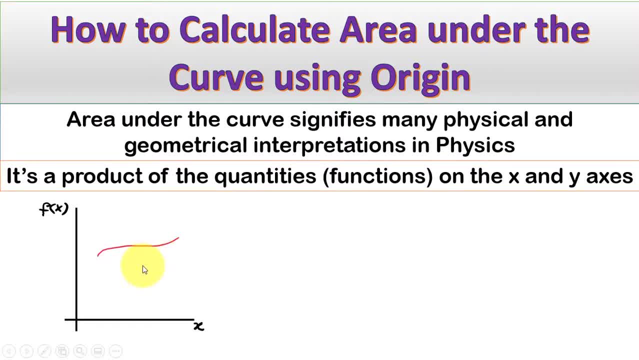 can remove this additional area by considering small rectangles. here i will cover this whole area under the curve with respective areas of the rectangles is a1, a2, a3 and a4 and the total area is equal to this. and in terms of f of x and x i can write it like this: now, here i see that a very small additional. 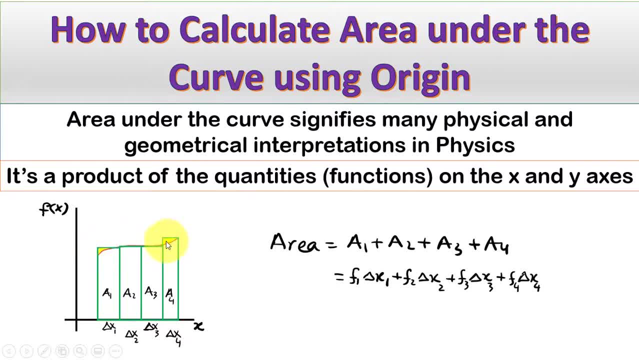 area is here, so i will have to eliminate this area as well in order to calculate the exact area under the curve. so what i can do, i will have to consider many small rectangles here and then i will have to eliminate that additional area calculation. the best i can do when i will. 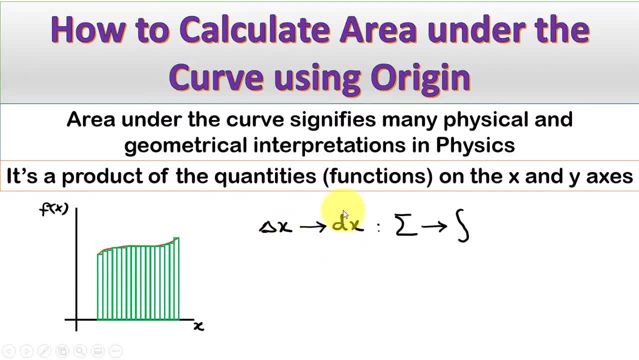 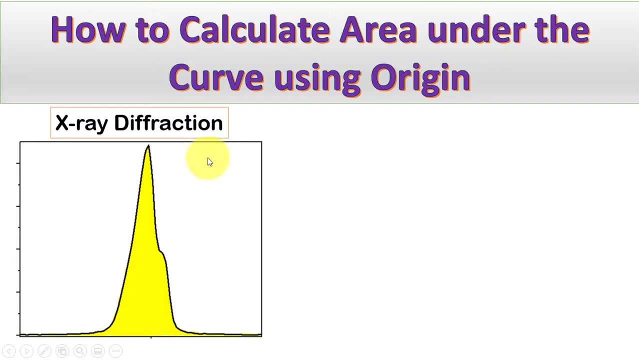 consider this delta x so small that it can be replaced with a differential x- dx. in that case the summation will go to integration and i will write area under the curve. you is f of x dx When I consider the x-ray diffraction and I am having this curve and I want to find out. 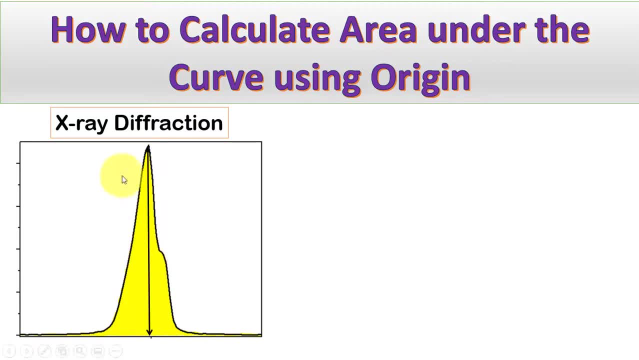 the area under this curve, As I know that height in xrd and the width in xrd are having their own importances, So the area is having the composite information about the crystalline state of the sample. As I know, that area under the curve will give me the total diffraction volume and it gives 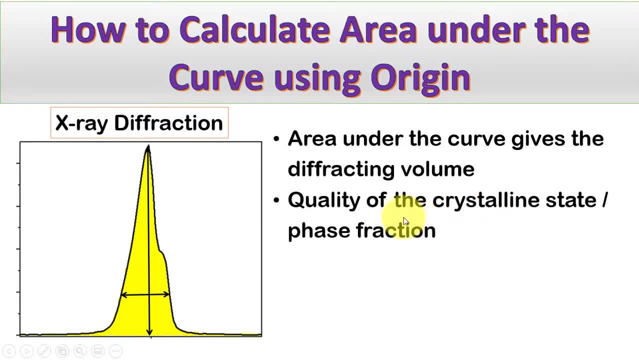 in other words the quality of the crystalline state, which we call is phase friction. Less area or sharp peak will indicate single crystallinity and the wider peak will be an indication of a polycrystalline state. Now, in order to find out the difference between the x-ray diffraction and the width in xrd, 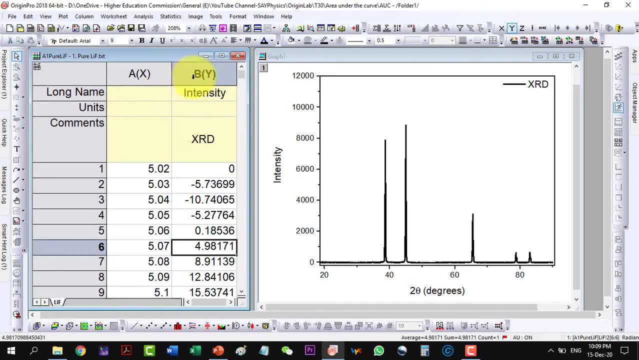 in order to calculate area under the curve. I am plotting this xrd data here. I will now find the area under these curves So I can focus on a specific curve or all the curves at the same time. So to find area under the curve I will have to go to analysis and then peak and baseline. 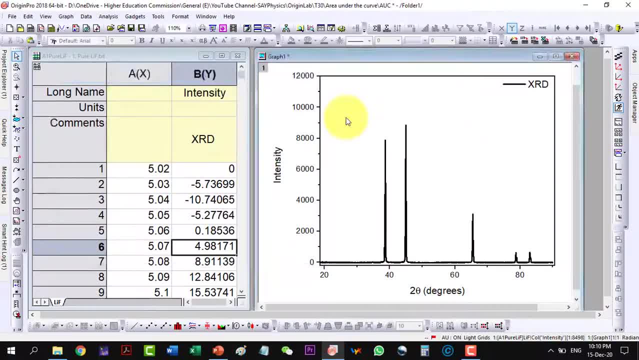 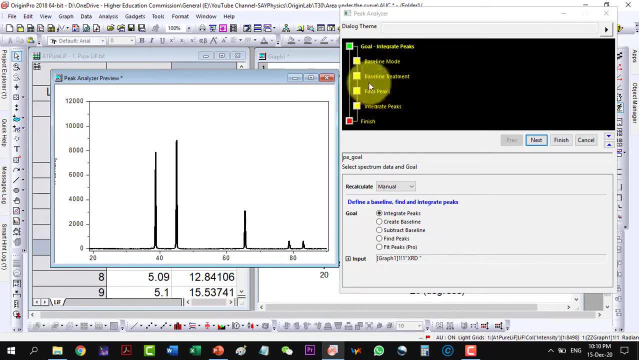 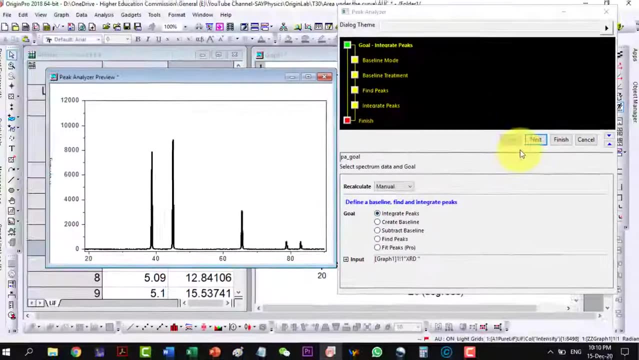 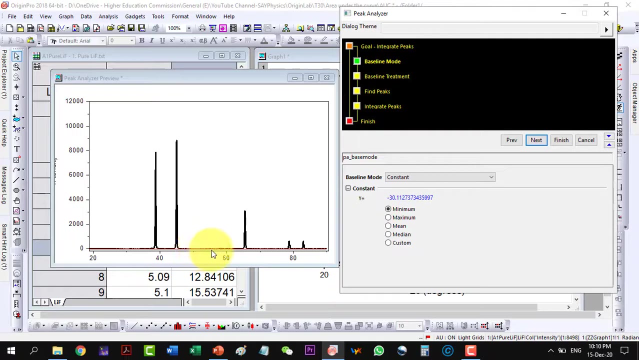 and to the peak analyzer and I will open the dialog. As I open the dialog, then a preview opens here which will give me indications as I go on with this menu. Now I am doing the integrate peaks, So I will click next and here the baseline mode. So the red line is shown here. It is the. 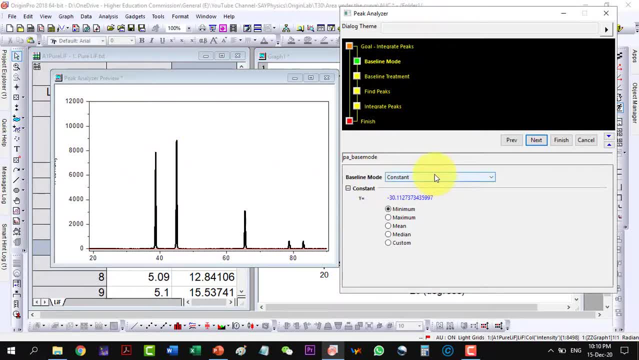 baseline. This is already baseline corrected data, So I will not do any change here and I will go to next and then I can click auto subtract the baseline because it is already having no effect on my data, and I will click next. It is saying that currently the number of peaks are zero, So I will have to find the peaks. 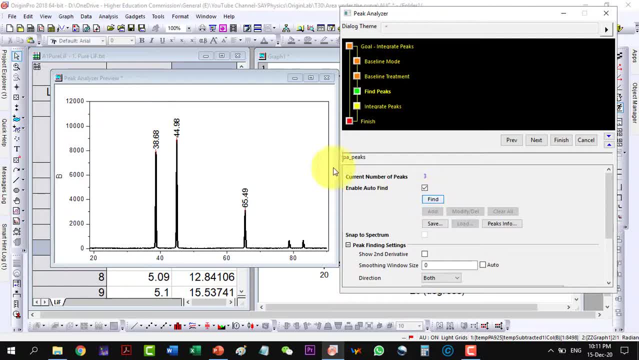 with the auto find and here they are. So it has found three peaks, as they are having the most of the contribution from these three peaks, While these two peaks are not auto found, so I can found them manually. But let's go on with these three.